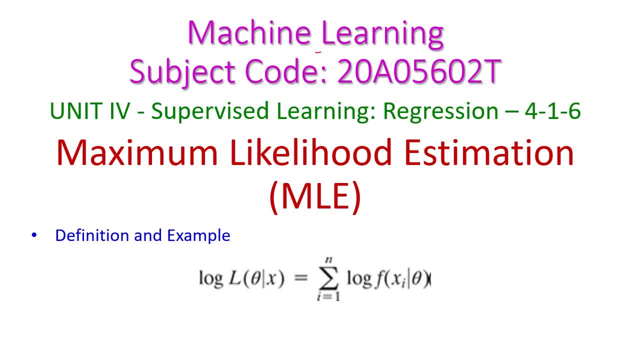 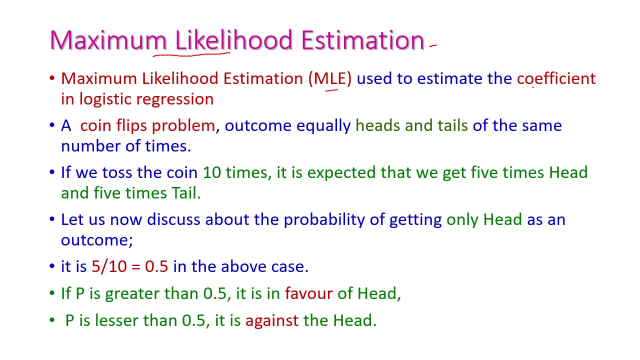 In this machine learning class we will see the maximum likelihood estimation, which is otherwise called as MLE, from fourth unit, supervised learning. This maximum likelihood estimation is the last topic from fourth unit and from the next class we will start our fifth unit. What is maximum likelihood estimation? That is MLE, So it is used to estimate the coefficient. 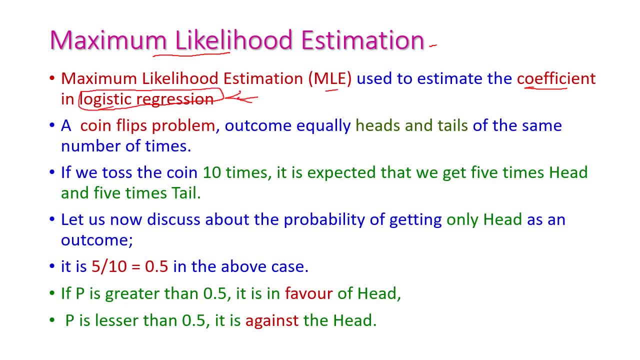 of logistic regression. So the coefficient will be either 0 or 1, isn't it for logistic regression? Let us take one problem, that is coin flip problem. Suppose, if we toss any coin we will get either head or tail. If we get head, then it is 1.. If we get tail, then this is 0.. 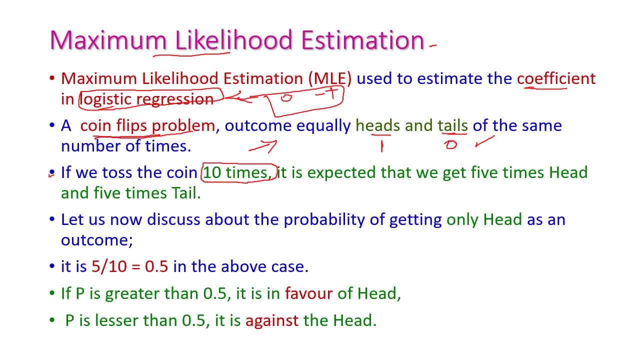 Suppose, if we toss the coin 10 times, then what is the expectation? It is 0.. So if we toss the coin 10 times, then what is the expectation? It is 0.. Expected outcome: 5 times we will get head and 5 times we will get tail. So this is what the 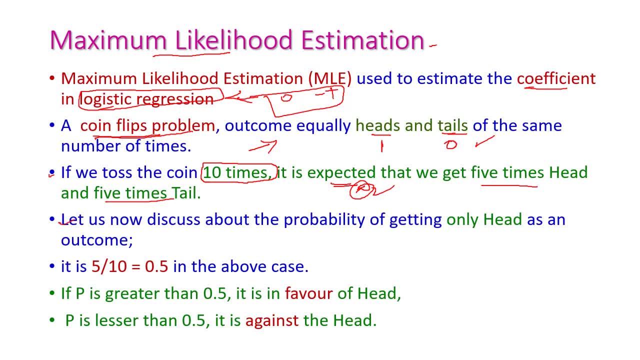 expected outcome: right. So now, what is the probability of getting only head? Okay, how many times we are tossing our coin? 10 times, How many? what is the expected outcome for getting head? That is 5,, isn't it So 5 by 10,, which is equal to 0.5. 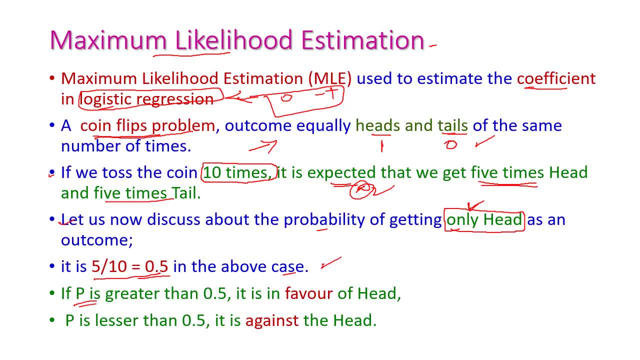 As per our our guess. Suppose if p value, that is, the probability value, is greater than 5,, that is, 0.5, then this is favor of head. Okay, Suppose if the probability value is less than 5,. 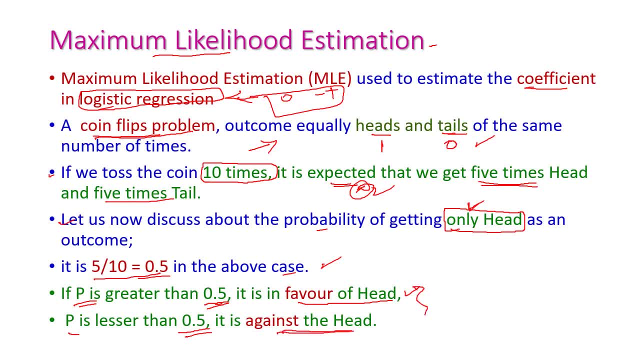 then this is against head. Okay, So our problem is: what is the probability of getting only head? We never talk about tail, right? So if the p value greater than 0.5, then favoring of head. If the value is less than 0.5, then this is against. 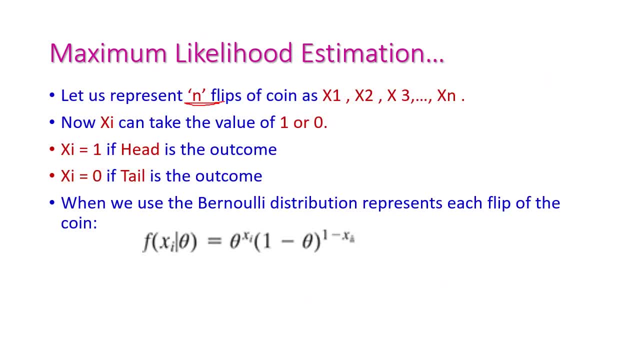 head. Suppose, if we flip n times of this coin, then x value equal to x1,, x2, etc. up to xn. That is n times we are going to toss our coin. Now xi can take any value: 0 or 1.. 0 means tail. 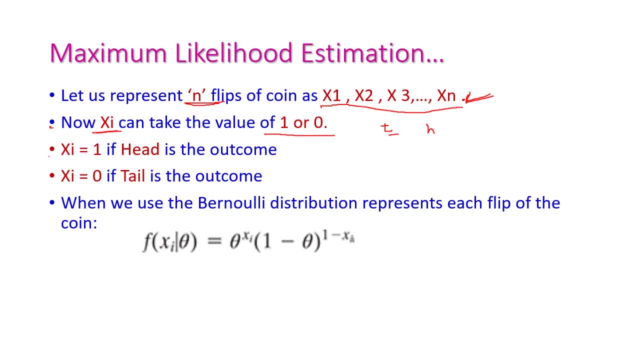 and 1 means head. Okay, If xi equal to 1, that is head is outcome. xi equal to 0, then tail is the outcome. Now we use the Bernoulli distribution, which represent each flip of the coin. that is flip. 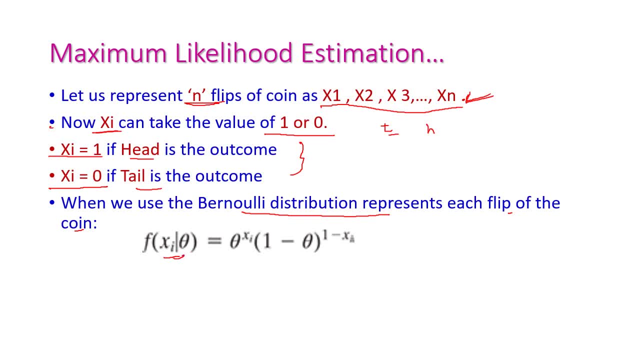 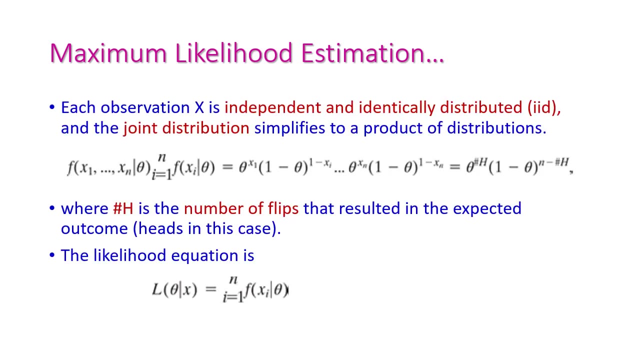 the f of xi, given theta, which is equal to theta power xi, into 1 minus theta, whole power, 1 minus xi. So this is the, the Bernoulli distribution equation. Here each observation x is iid. iid means independent and 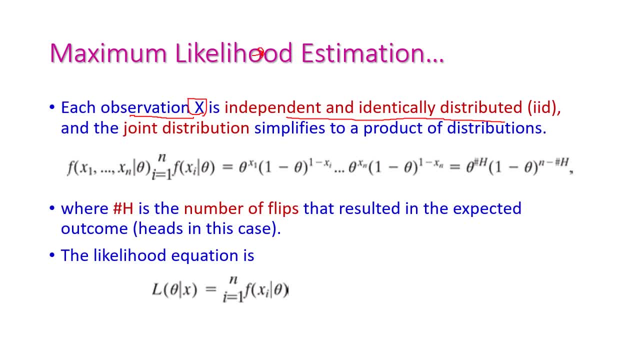 identically distributed. That means each flip is independent to each other. Okay, So this is different. In this flip, we will get either 0 or 1.. And in this flip, we will get either 0 or 1,. 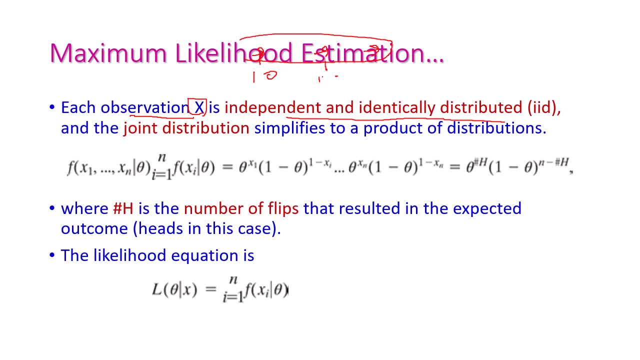 that is head or tail, head or tail. Okay, So these flips, that is x values or iid, that is independent and identically distributed, And the joint distribution simplifies the product of distributions. product of distributions, that is f of x1 to xn, which, given theta. 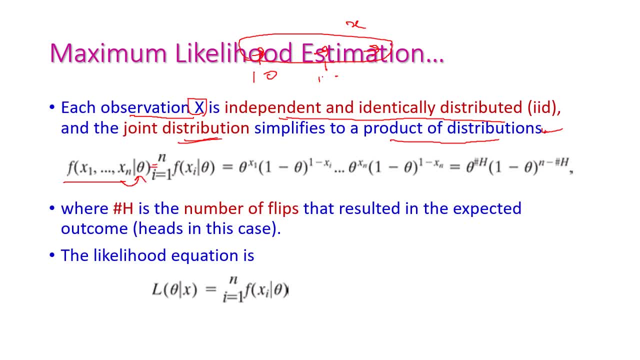 which is equal to i, equal to 1 to n, f of xi, theta That is x equal to x1 to xn, is simplified into xi. Okay, Equal to theta of x1 into 1 minus theta of 1 minus xi, etc. up to theta of x, power n into 1 minus. 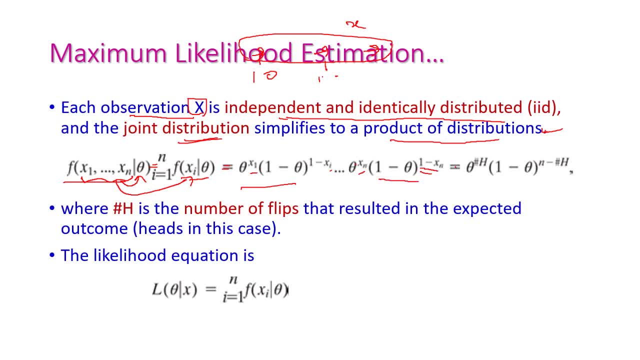 theta whole power 1 minus xn, Okay, Which is equal to theta power, hash i of 1 minus theta whole power, n minus hash i. Okay, This is the simplified formula, And hash h is nothing but the number of flips that resulted the expected outcome. So, as per our example, the expected. 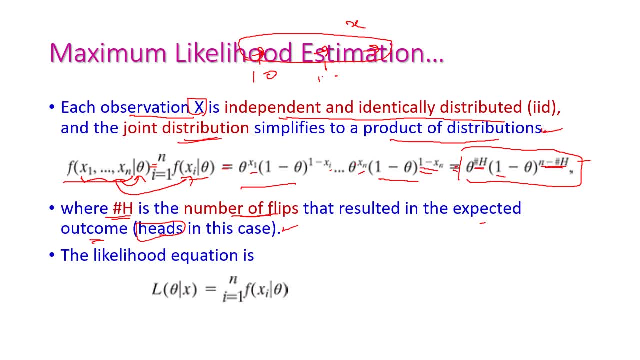 outcome is head. Okay, Now the likelihood equation is likelihood l of theta gives x. This is the likelihood: theta gives x, which is equal to i, equal to 1, to n, f of xi, given theta. So this is the likelihood equation, But the likelihood function is not a probability.